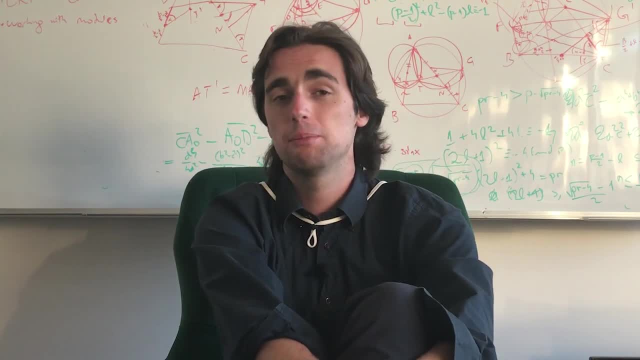 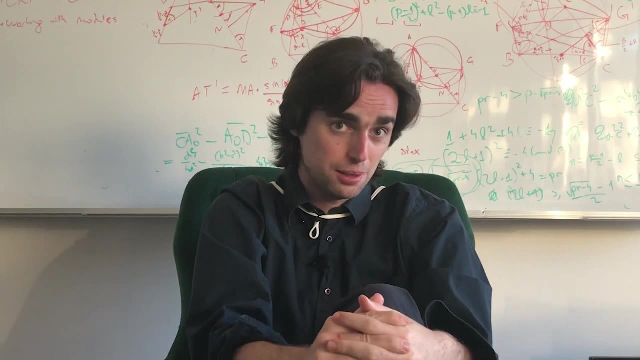 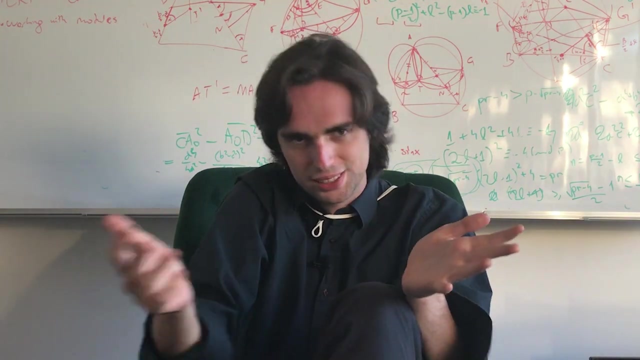 Hello, fellow problem solvers. So today we're going to be talking about the combinatorics that you need for the International Math Olympiad. How do you learn it? So now, without further ado, let's begin. As always, what you need to do is you need solve problems in combinatorics. This is true for every. 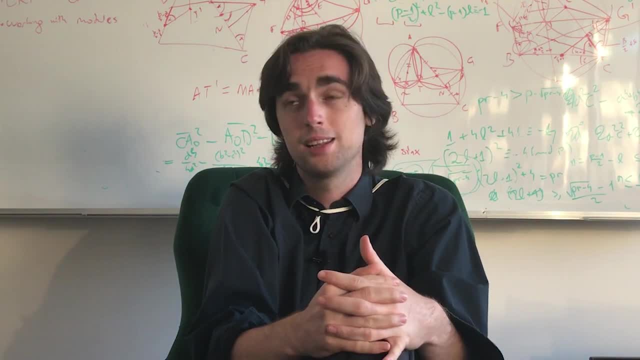 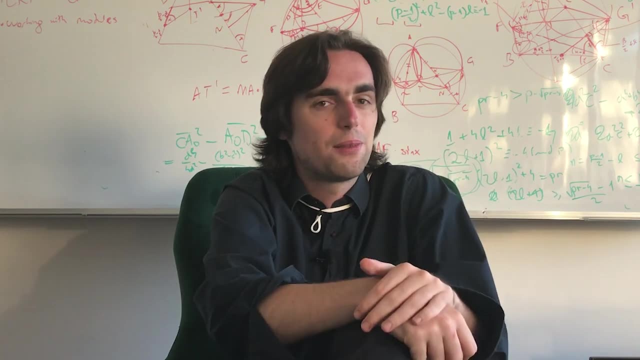 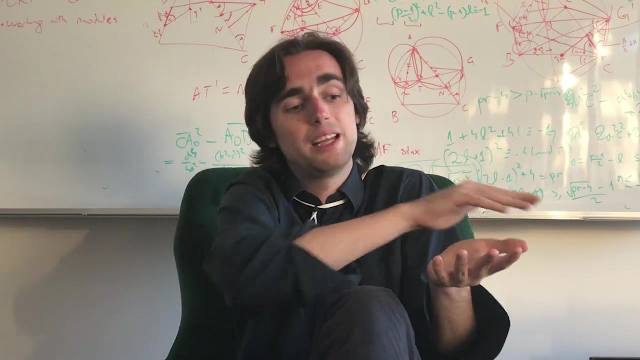 single one of these four fields that are at the International Math Olympiad. And with combinatorics there is an element of problem-solving. like you, Combinatorics at the beginner level is about turning words into equations and then solving them. That's what it is at the beginning, But later on it becomes much. 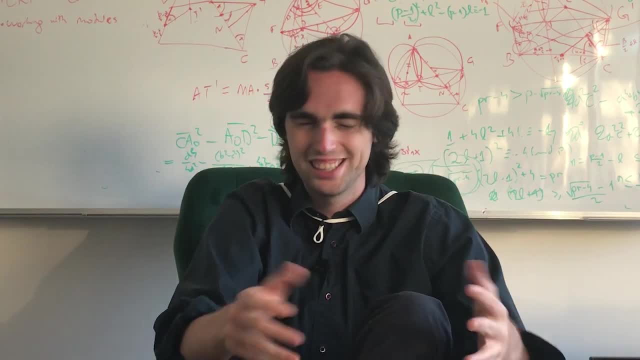 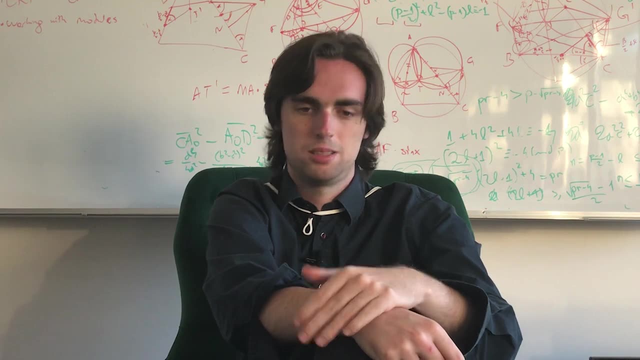 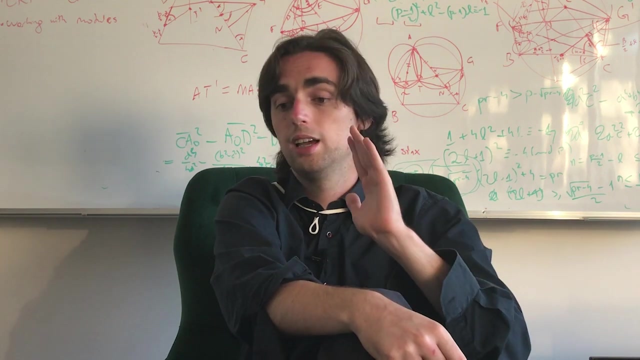 more than that, It becomes very interesting. It can be games that you learn how to play and how to find winning strategies. You know if, if there is, say, eight coins on a pile and at each turn you and I we're gonna play alternately. 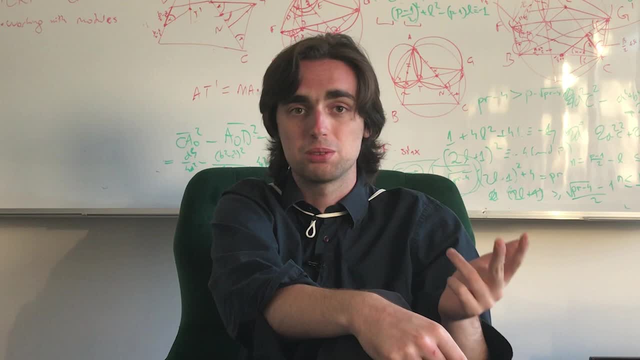 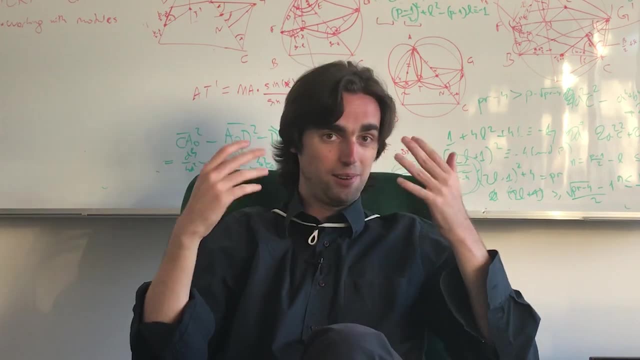 And at each turn you can take one, two or three coins from the pile. Who's going to win? Would you like to play first or second? And these types of problems can get very, very interesting and very, very cool and can have a vast. they cover a. 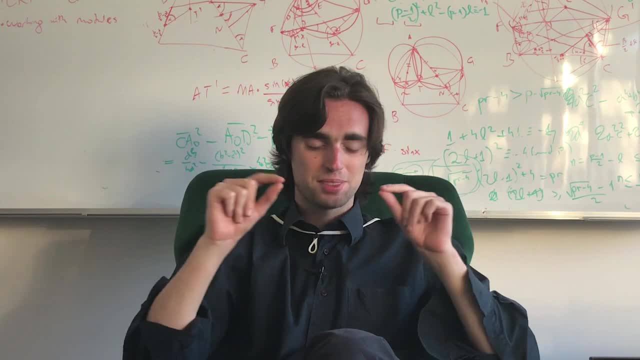 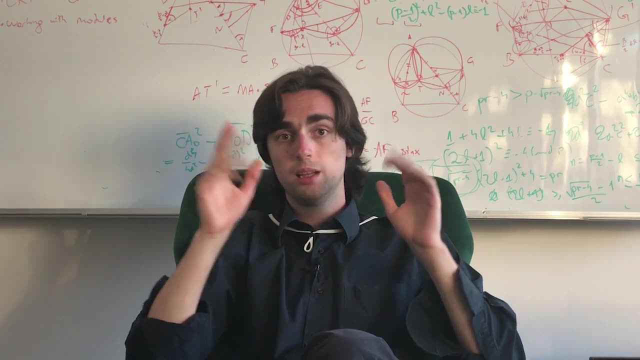 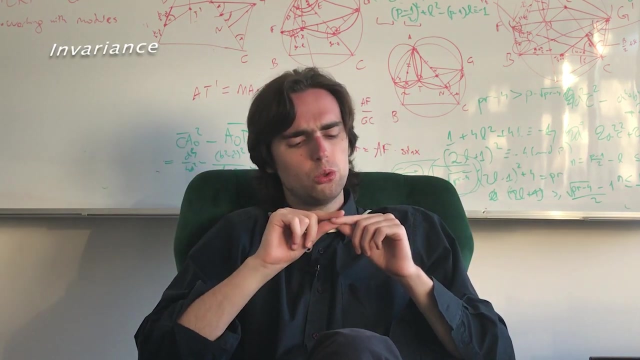 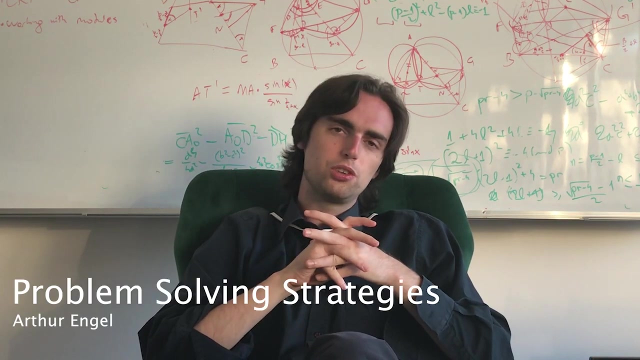 vast area of mathematics. So now here's the things you should look for in books that cover combinatorics. Number one is: you really need to learn about the invariance principle, And I'll say, actually I'll mention two good books for this. One is sort of an introductory type, maybe intermediate level book, which is 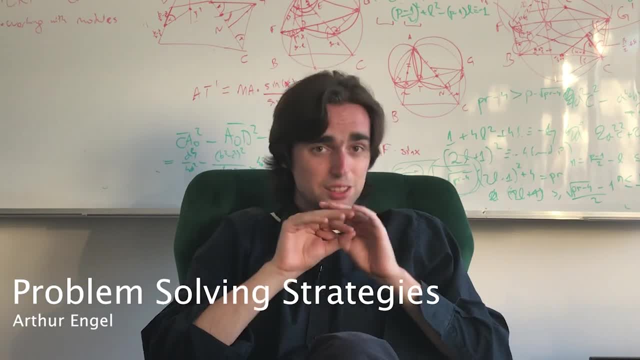 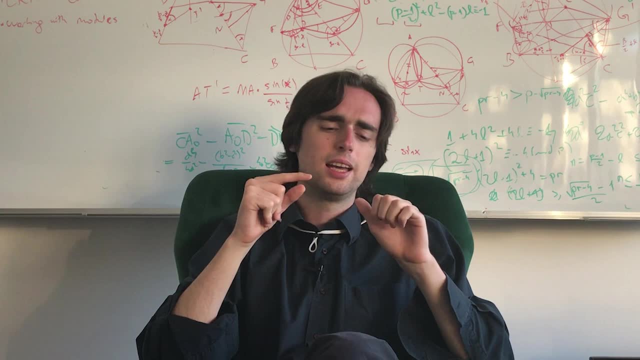 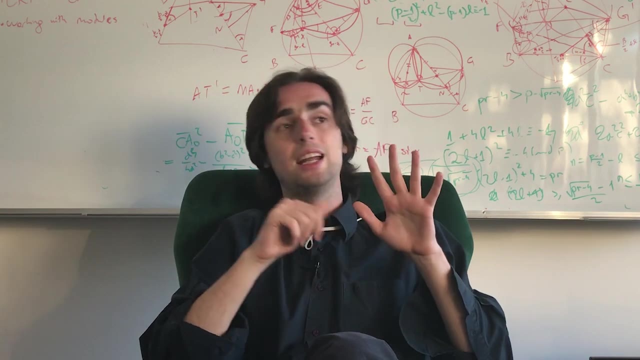 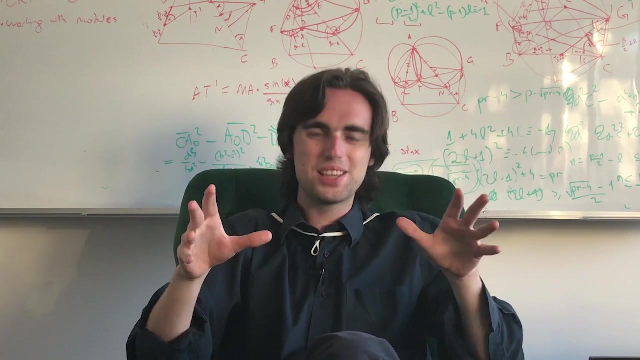 problem-solving strategies by Engels. This book is amazing for combinatorics, for teaching you some basic principles: Coloring proofs, the box principle, invariance, the extremal principle, induction and games. These six things are very common principles in combinatorics. They're very 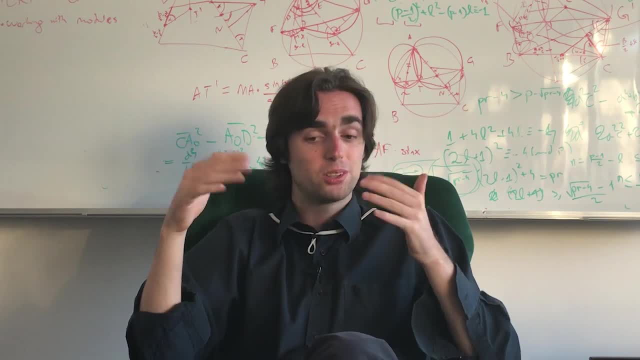 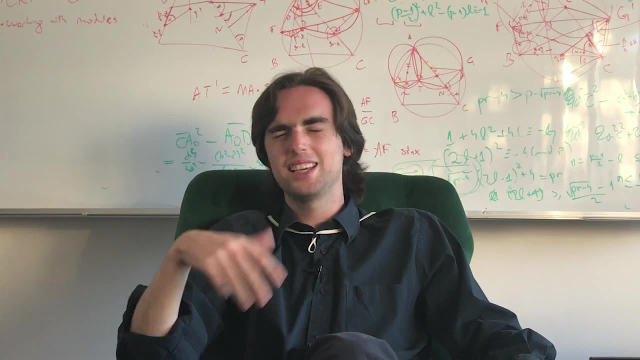 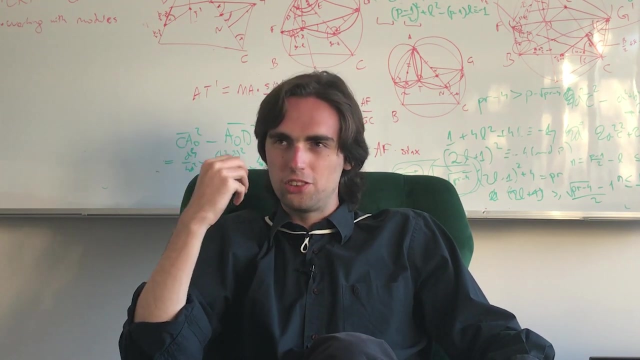 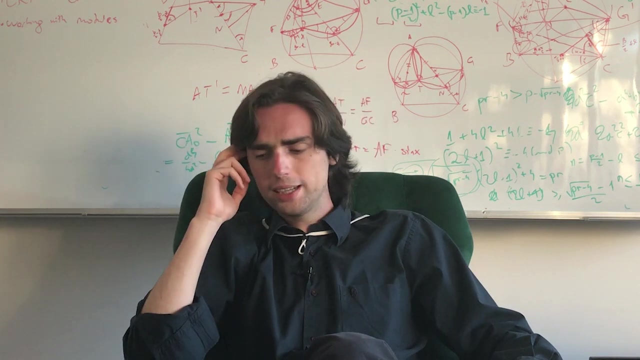 useful That really many combinatorics problems are just them applied to more difficult and more interesting ways, And sometimes these problems that are difficult actually are an ingenious way or creative way of you using one of these principles. So that's one book I would recommend. Another one is called the 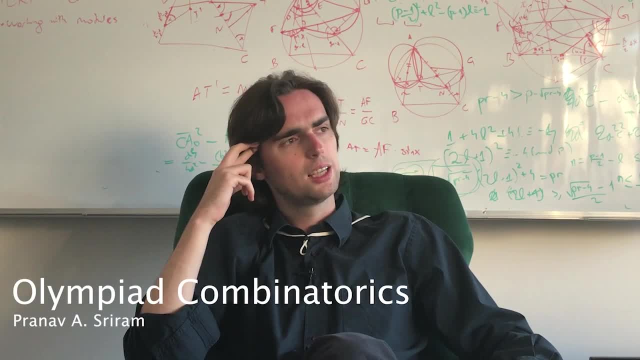 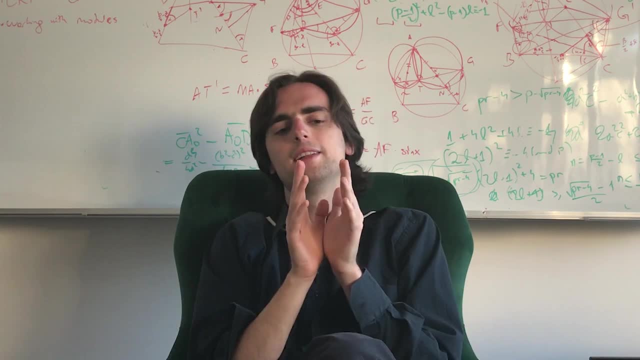 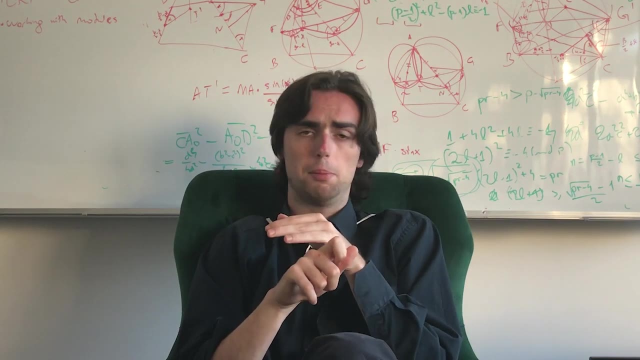 Olympiad Combinatorics by Pranav Sriram, I believe, is the name. I'll link the book in the video description. And that's a book which covers algorithms, games, graph theory, even covers the probabilistic methods, which is not used very often, but 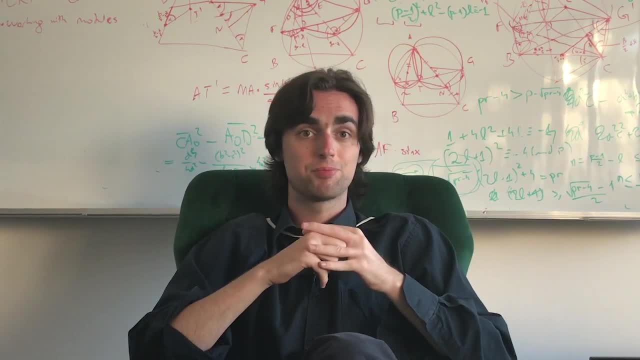 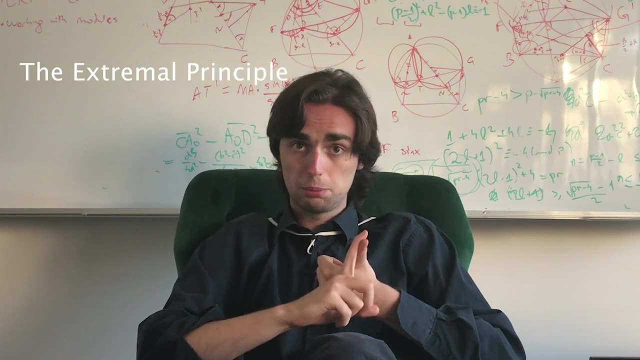 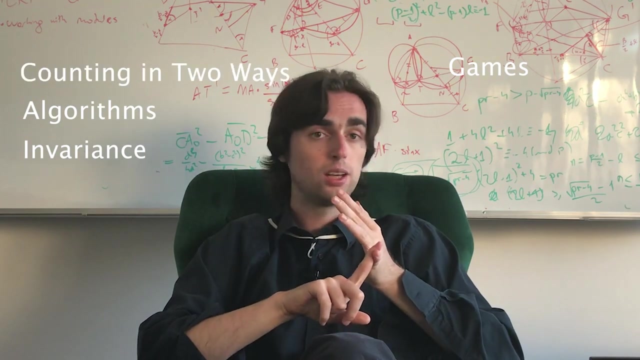 it can be useful sometimes in math competitions. So those are the two books. Now what you really need to look for, look for is the extremal principle: algorithms. invariance teaches you something about games, double counting or counting things in two different ways. graph theory- at least a little bit. 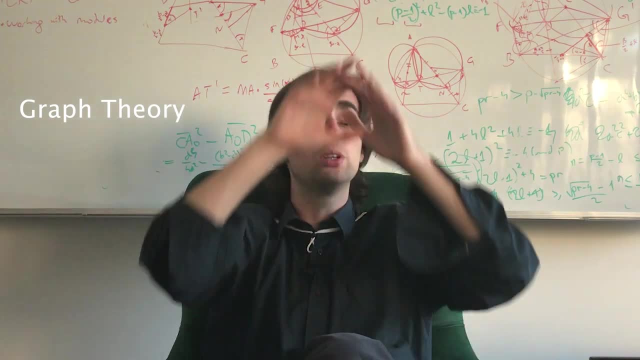 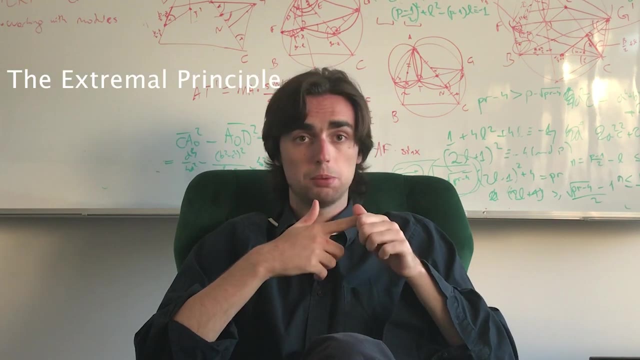 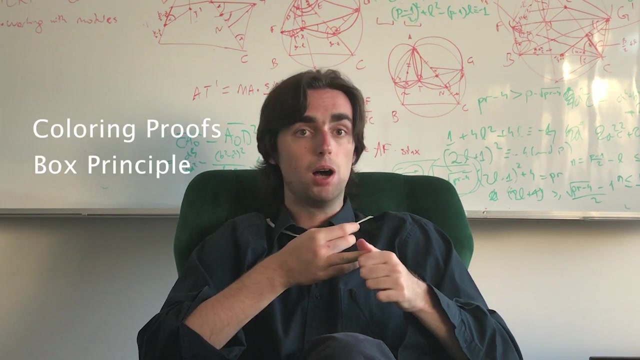 so you have some basic understanding of what it is, because you can look at a lot of problems from graphs. other than that, there is the extremal principle, applied in many different ways, and that i believe is oh, coloring proofs, and the box principle or the pigeonhole principle. 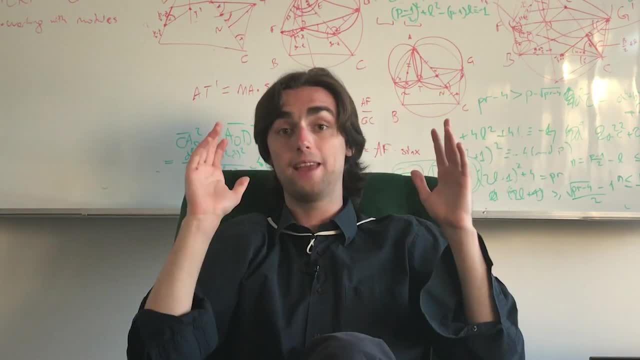 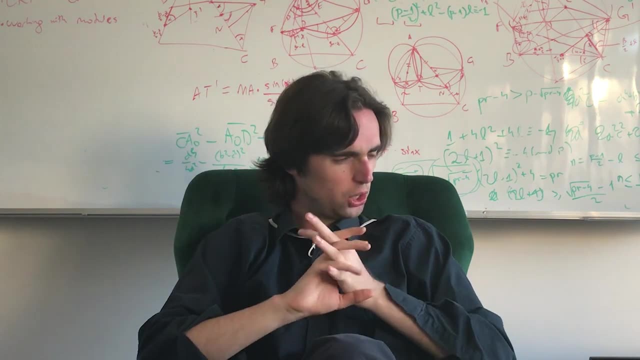 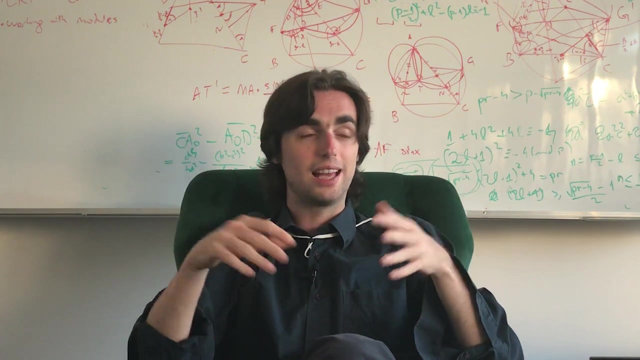 that can be applied in so many different ways: shapes and forms. and finally, i'll mention that you need to learn how to use induction, because there's a quote that i heard- i'm not sure if it was by gauss or someone else- but a mathematician is only as good as they know how to use induction, which i think is pretty cool. 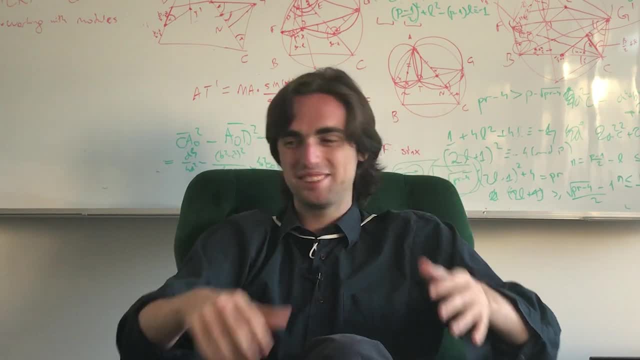 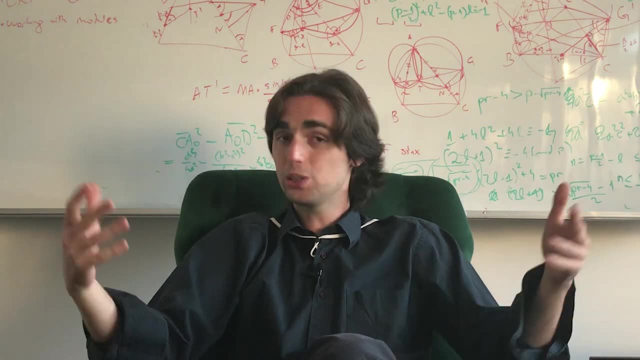 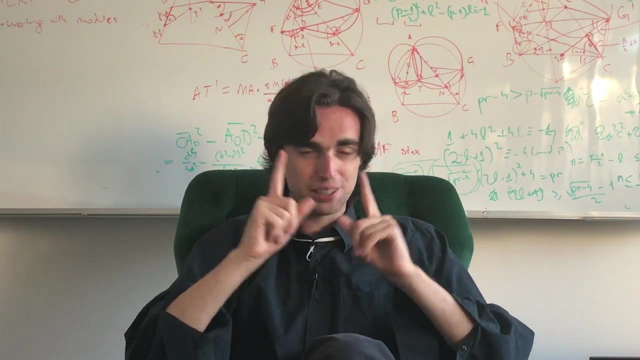 and sometimes the problems. you really see that so you can use induction in very, very, very creative ways. that's really all you need for combinatorics now after you've done that. it's about problem solving, and a great competition to solve problems in combinatorics is the 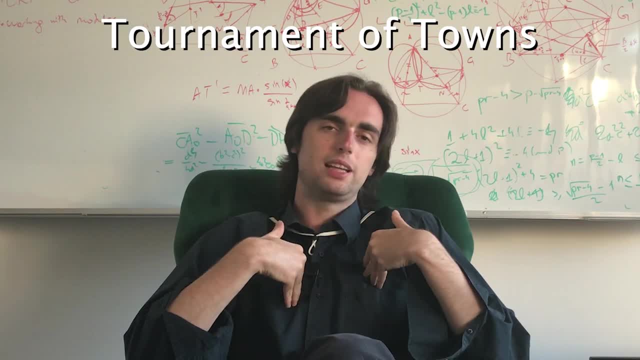 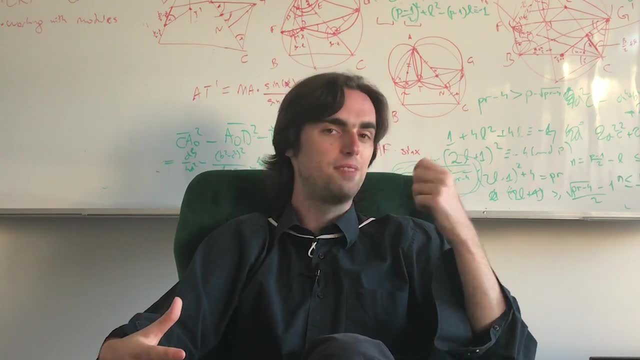 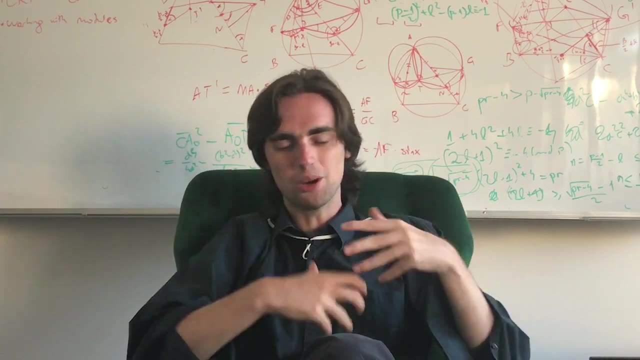 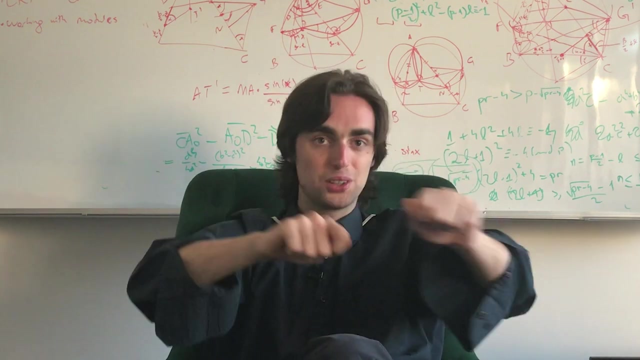 tournament of talents. i, i personally enjoy those problems very, very much because they don't require so much theory, but they're very smart. sometimes they're so good because, like, you're losing really just thinking, and combinatorics is about that. it's about you trying to solve problems at the most basic level. you're looking at different.